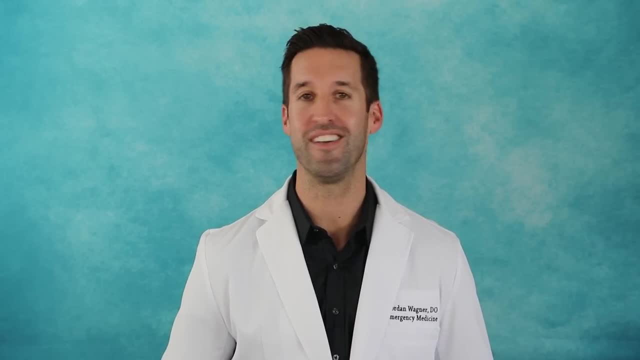 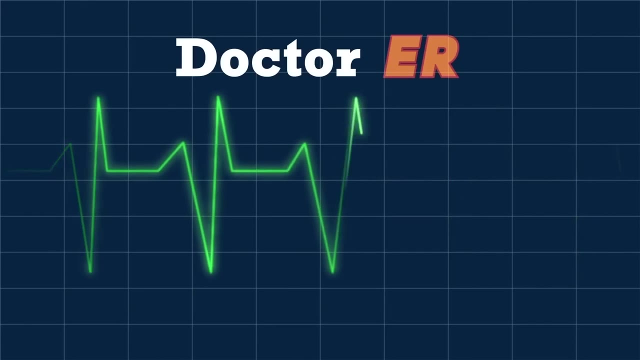 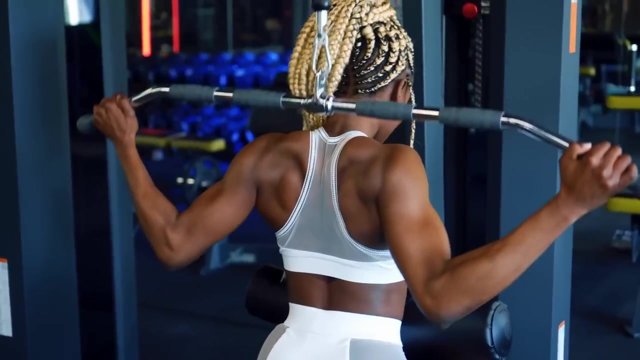 All men are created equal, but your protein powder is not. Say what Yep. So what is the best type of protein powder? Athletes and individuals who regularly lift weights may find that taking protein powder helps maximize muscle gain and increase fat loss, But that's. 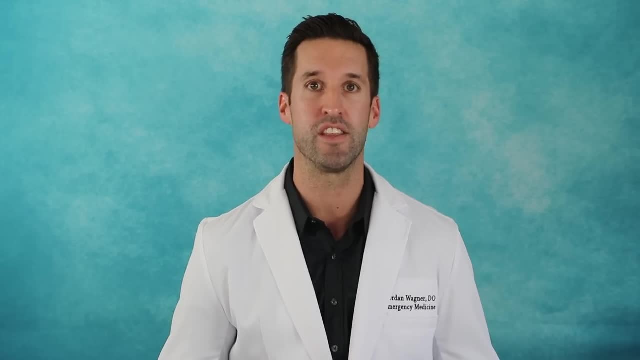 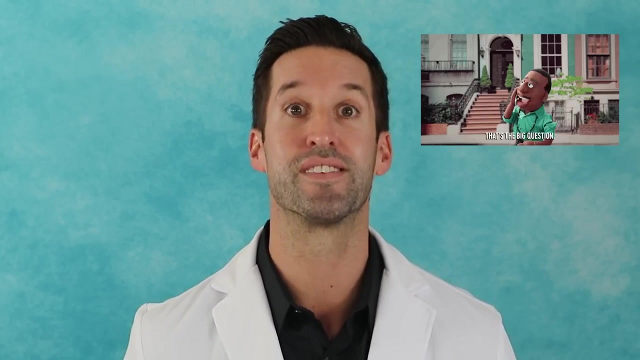 not all my friends. Protein powders can also aid individuals such as people who are ill, older adults and some vegetarians or vegans who struggle to meet protein needs with food alone. So, all that being said, which type of protein powder is the best? This is the big question. 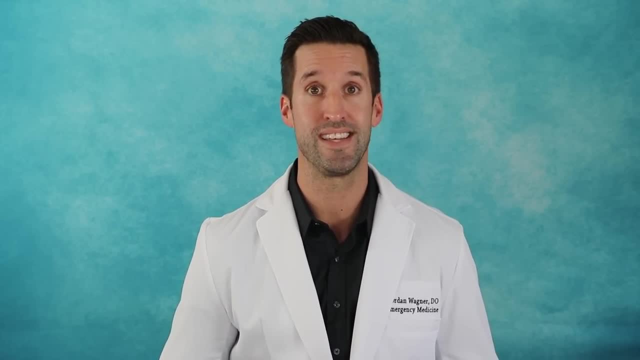 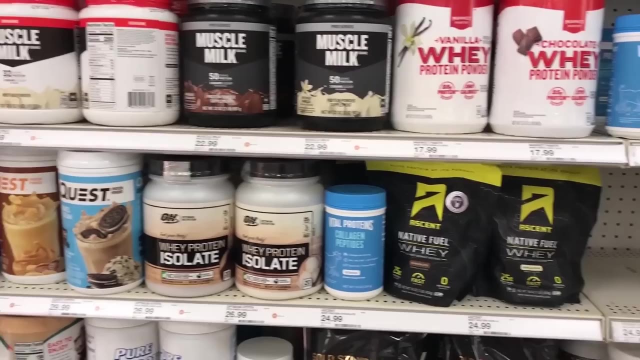 Let me first say the number one option for getting your protein needs should come from the food in your diet. There are an infinite number of protein powders on the market made from a variety of sources. It can be difficult to determine which protein is right for you. 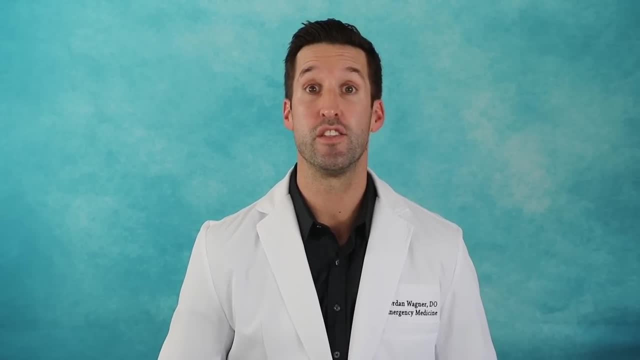 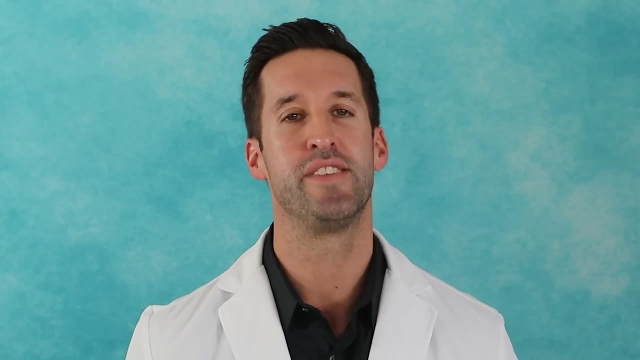 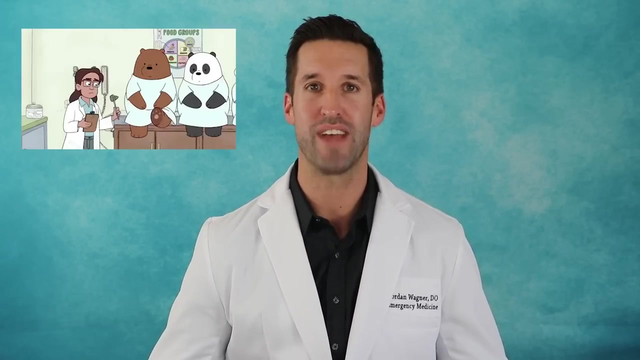 That's why, today, I'm breaking down everything that you need to know about the top five types of protein powders out there. This is based on your desired fitness results, dietary preferences and lifestyle, So stay with me, Hey everyone. I'm Dr Jordan Wagner. I'm an emergency room doctor who treats 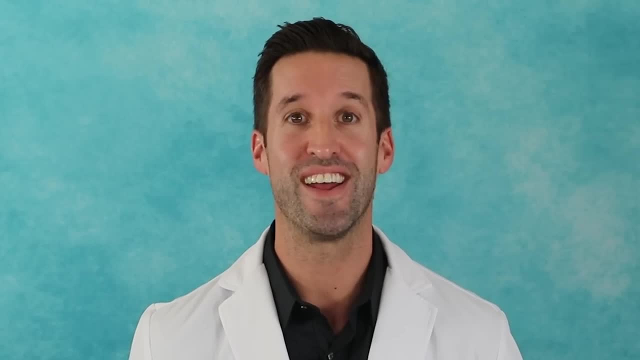 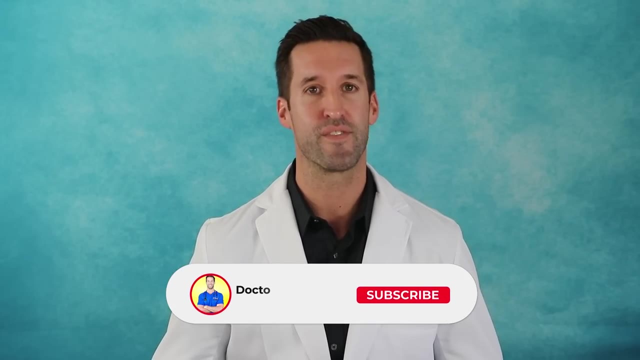 everything from COVID to gunshot wounds, burns, you name it. I've created this video series to help answer some of your medical questions and the questions that I get from patients each and every day. If you find this video helpful, please do me a favor and subscribe. 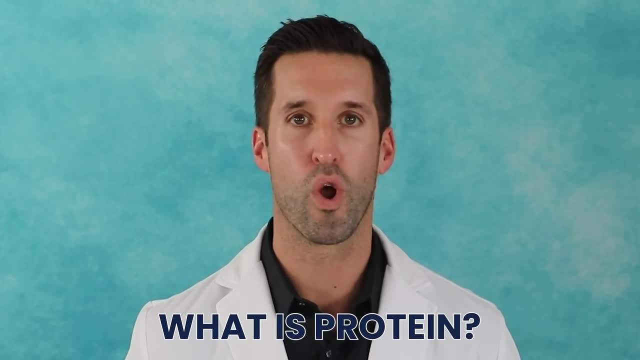 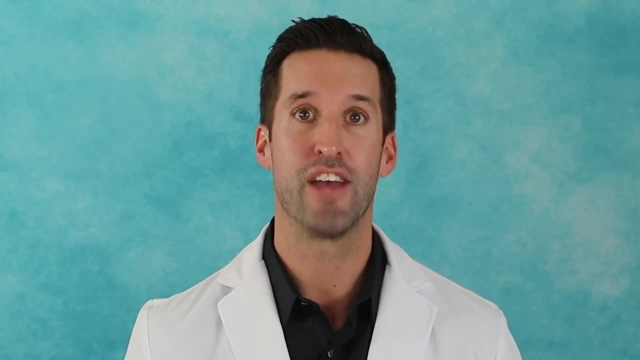 First things first. let's understand What in the world is protein and why does our body need it? Well, on a basic level, your body needs protein to stay healthy and to work the way it should. Protein is found literally in everything from your organs to your muscles, your skin. 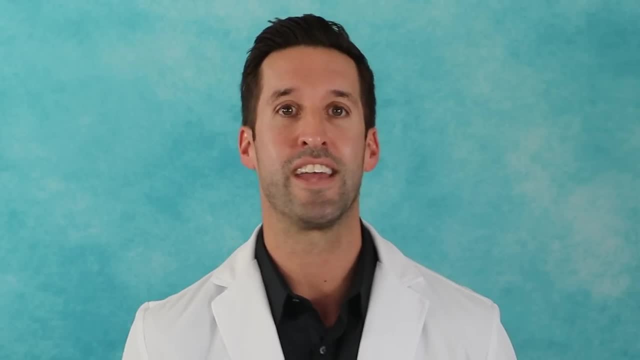 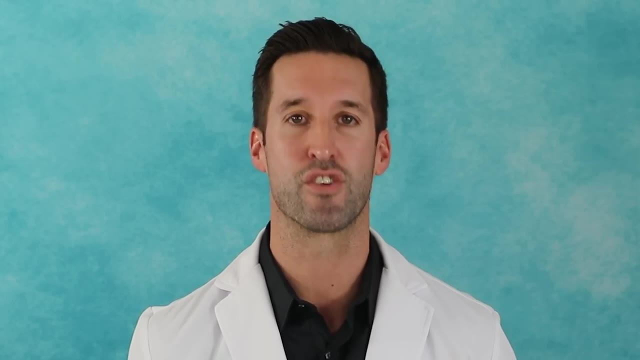 hair, tissue, bones, And it also plays a major role in carrying oxygen throughout your body, in your blood, and it helps fight off infections, keep cells healthy, and the list goes on and on. If you aren't getting enough in your diet, this can lead to muscle loss. 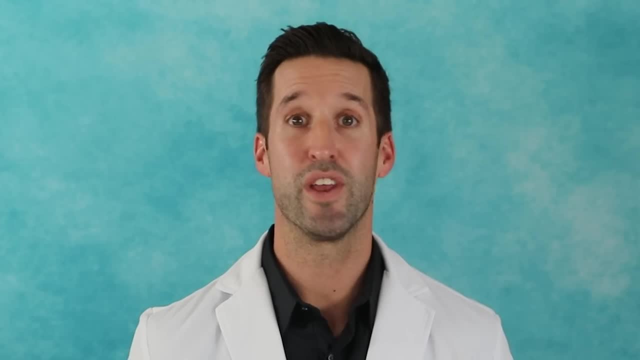 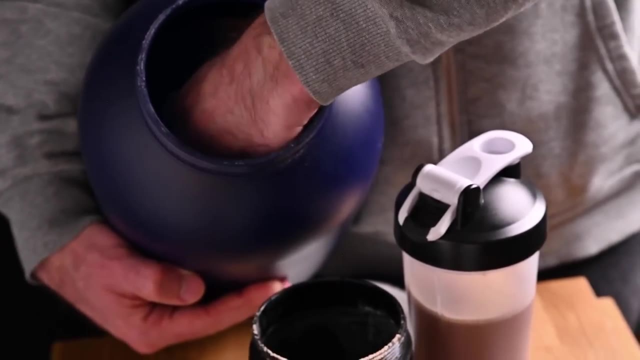 tissue breakdown and all sorts of other health problems, And we don't want that. So a great way to supplement protein in your diet is to get it through means such as a protein powder. Protein powders are concentrated sources of protein made from either animal or plant foods. 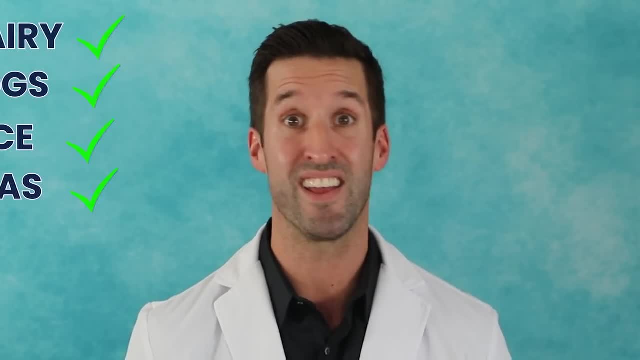 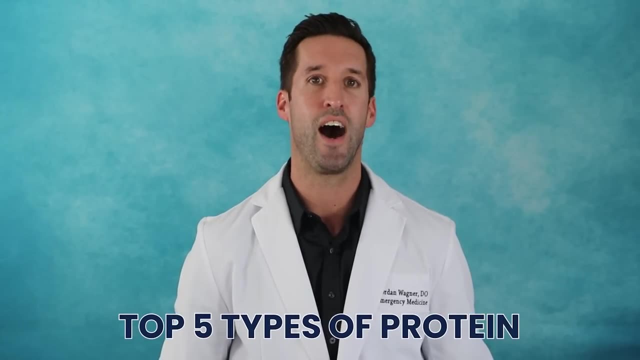 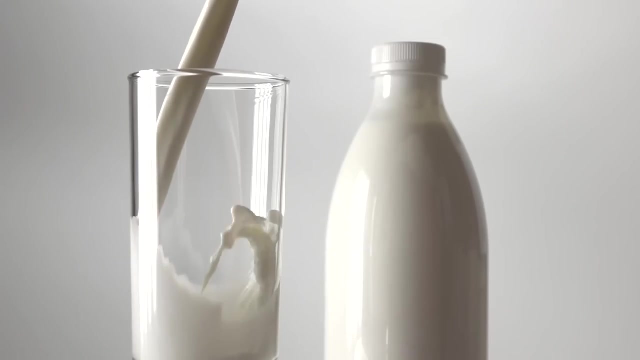 such as dairy eggs, rice or peas and many others. To take protein powders, you simply mix the powder with water or another liquid of your choice and consume. Here are the top five types of proteins on the market. Number one: whey protein. Whey protein comes from milk. Milk harbors lactose. 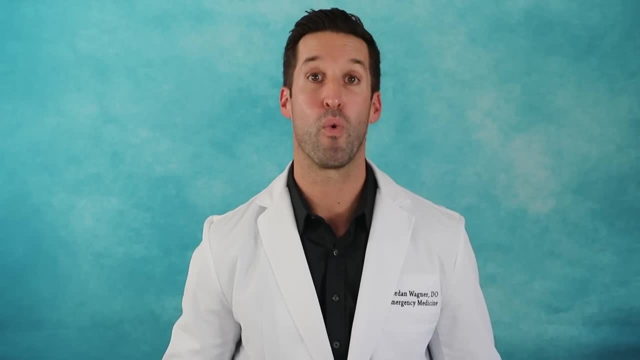 which many individuals have difficulty digesting. But while whey protein concentrate retains some lactose, the isolate version contains very little because most of this milk sugar is lost during processing. Hear that again. The isolated version contains very little because most of this milk sugar is lost during processing. Whey digests quickly and is rich in branched chain. 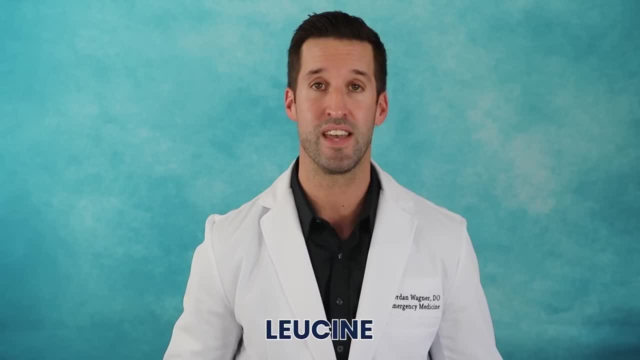 amino acids. Next is BCAAs- Leucine. one of these BCAAs plays a major role in promoting muscle growth and recovery after resistance and endurance exercise. When amino acids are digested and absorbed in your bloodstream, they become available for muscle protein synthesis. NPS or the creation of new muscles. Studies reveal that whey protein can help build and maintain muscle mass, assist in athletes with recovery from heavy exercise and increase muscle strength in response to strength training. One study in the Journal of Applied Physiology. 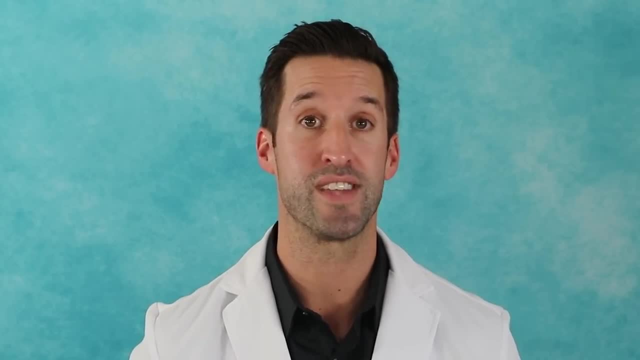 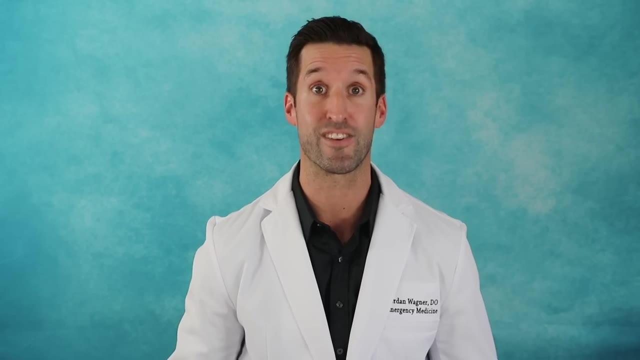 reported that 3% of those proteins are produced in muscle growth, but they're only produced in that. young men showed that whey protein increased MPS 31% more than protein and 132% more than casein protein following resistance exercise. Other studies in normal weight overweight. 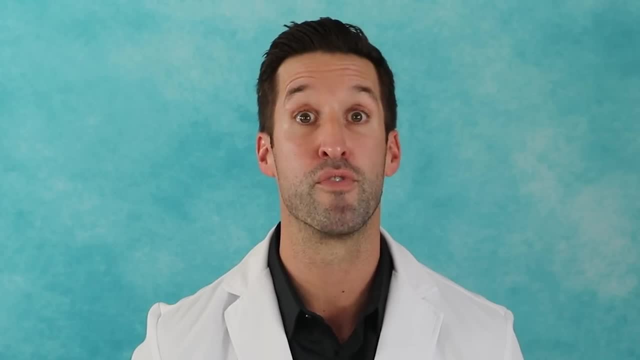 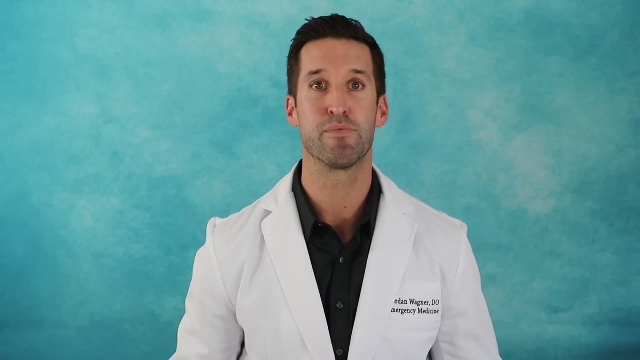 and obese individuals suggested that whey protein may improve body composition by decreasing fat mass and increasing overall lean mass. What's more, whey protein seems to reduce appetite at least as much as other types of protein. Some studies even suggest that whey protein 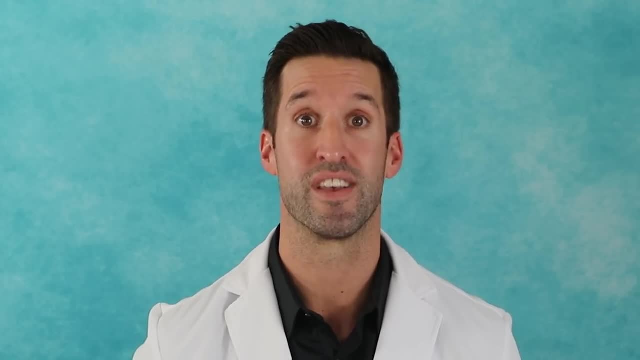 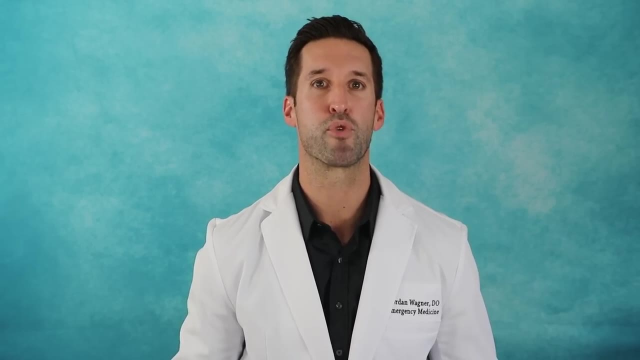 may also reduce inflammation and improve certain heart health markers in overweight and obese people. Number two type of protein: casein protein. Similar to whey. casein is a protein found in milk. However, casein is digested and absorbed much more slowly. 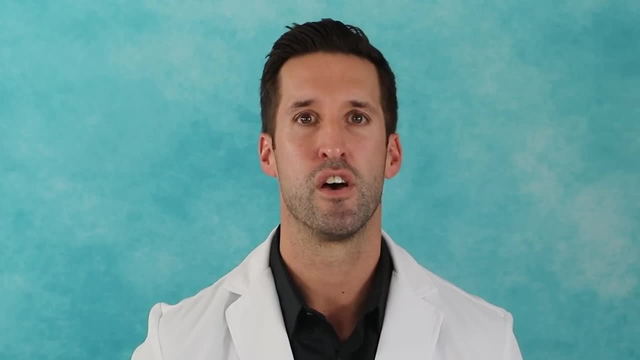 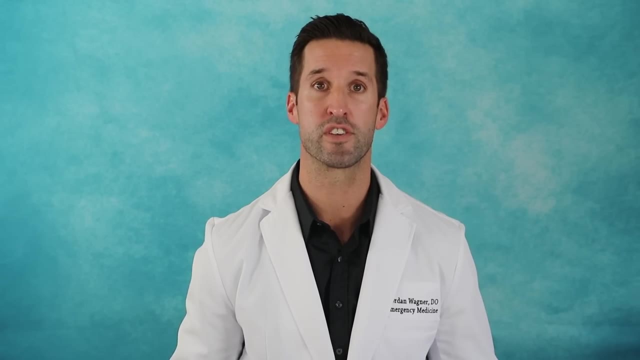 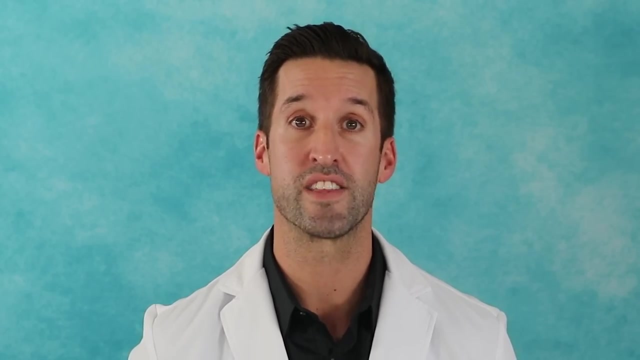 Casein forms a gel which interacts with stomach acid, slowing down stomach emptying and delaying your bloodstream's absorption of amino acids. This results in a gradual, steadier exposure of your muscles to amino acids, reducing the rate of muscle protein breakdown. Research indicates that casein is more effective. 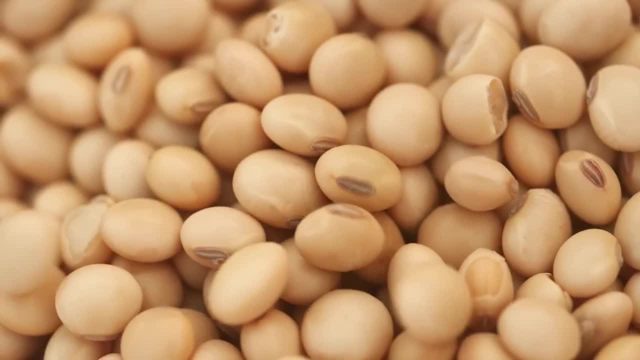 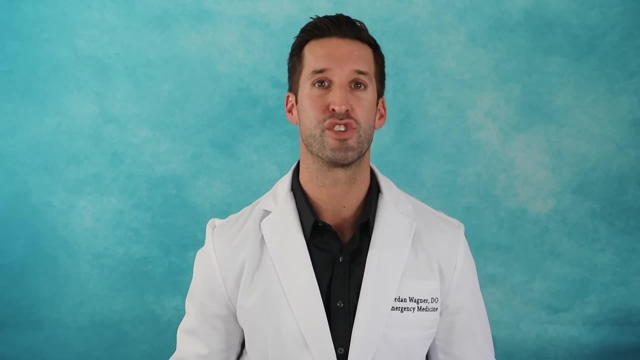 in increasing muscle protein synthesis and strength than soy or wheat protein, but less than whey protein. One study out of the Annals of Nutrition and Metabolism reported that overweight men suggested that when calories are restricted, casein may have an advantage over whey. 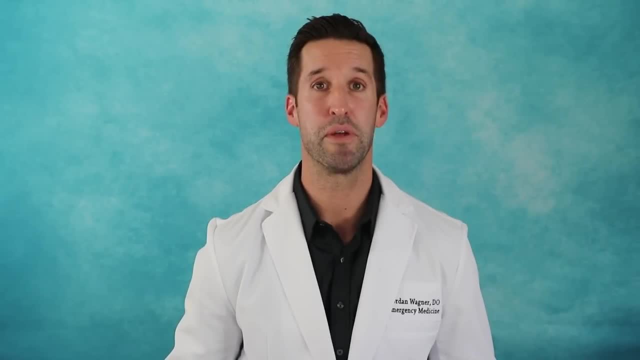 in improving body composition during weightlifting. Number three: protein option: egg protein. Eggs are an excellent- or should I say egg-cellent- source of high quality protein and fat. In fact, whole food eggs have the highest protein digestibility corrected amino acid score. 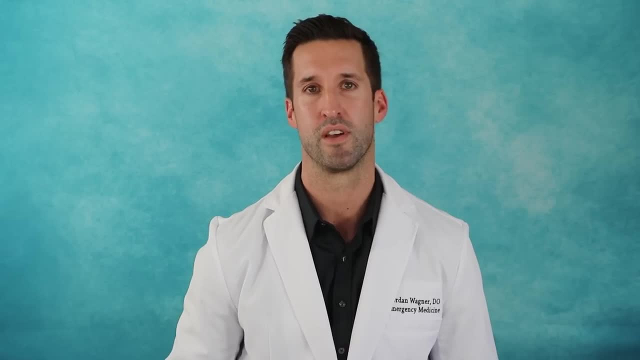 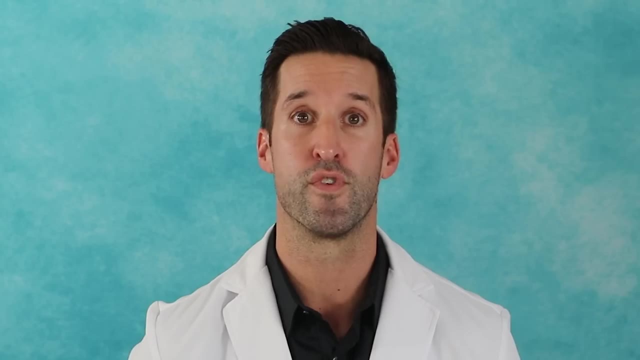 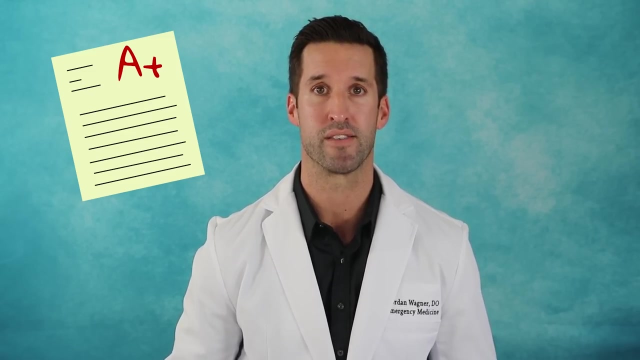 Like all animal products, eggs are a complete protein source. That means they provide all nine essential amino acids that your body cannot make itself. Eggs are also one of the best foods for decreasing appetite and helping you stay full for longer. That's why the protein quality remains at an A plus. 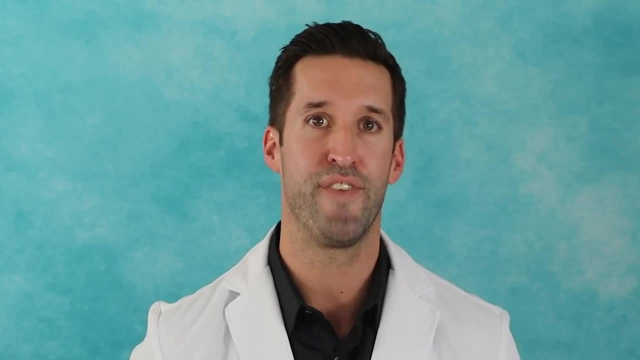 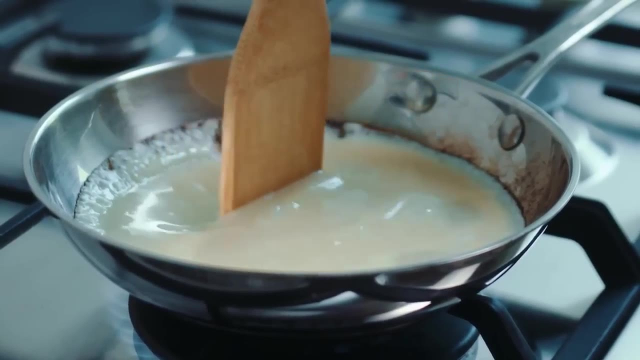 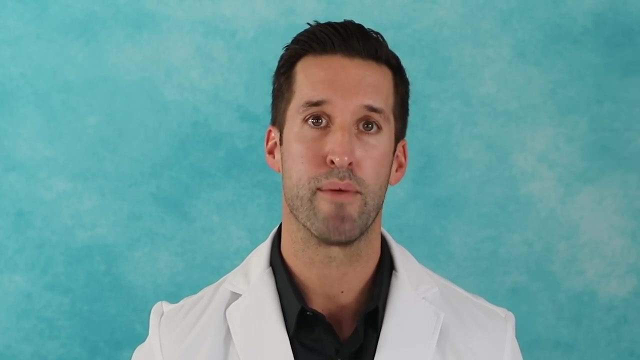 However, you may experience less fullness because the high fat yolks have been removed, resulting in just egg whites. Egg white protein could be a good choice for people with dietary allergies who prefer a supplement based with animal protein, but please keep in mind that egg white protein 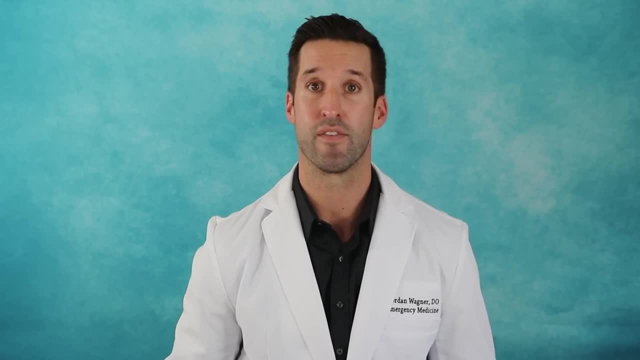 hasn't been studied as much as whey or casein. In one study out of the Journal of Nutrition, egg protein demonstrated less potential to reduce appetite than casein or pea protein when consumed before a meal. Number four: pea protein. Pea protein powder is especially popular. 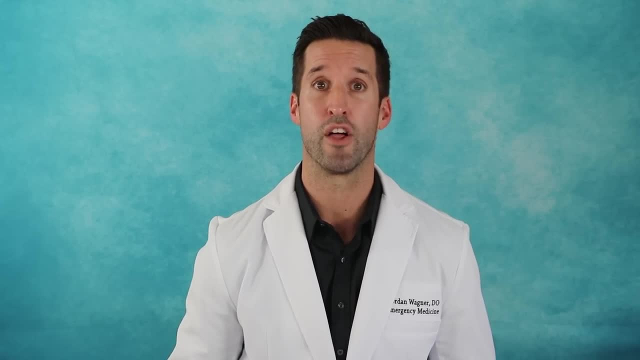 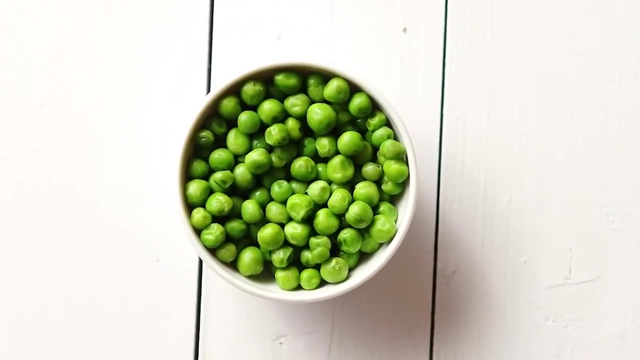 among vegetarians, vegans and individuals with allergies or sensitivities to dairy or eggs. Pea protein consists of split pea, a high fiber legume that boosts all but one of the essential amino acids. Pea protein is also particularly rich in BCAAs. 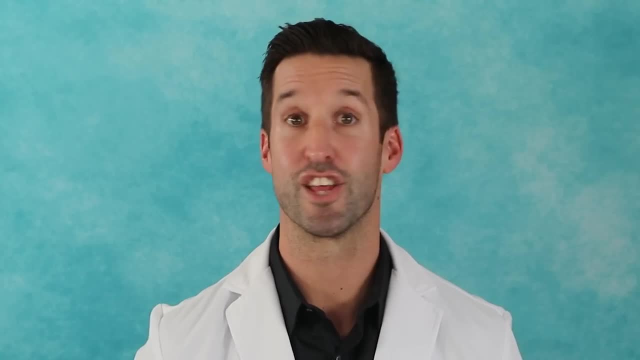 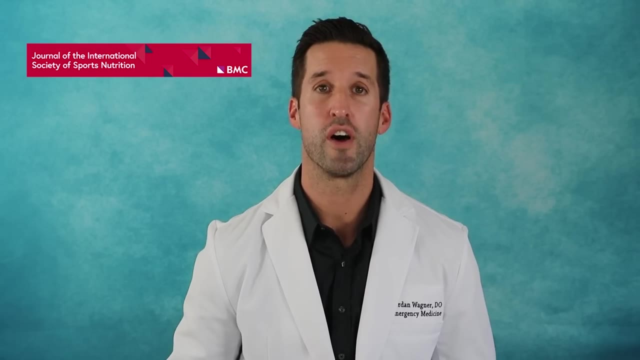 However, full disclosure. good tasting varieties are just a little tricky to come by, but I'll be sure to put a link to some of my favorites in the description below. So, when it comes to pea protein, the Journal of the International Society of Sports Nutrition. reported in a 12-week study in 161 men during resistance training, those who took 1.8 ounces, or about 50 grams, of pea protein daily experienced similar increases in muscle thickness as those men who consume the same amount of whey protein daily. 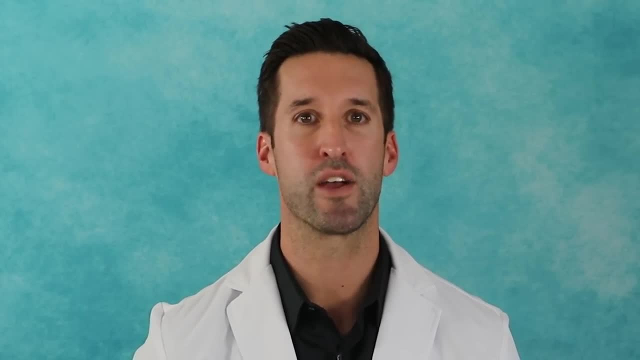 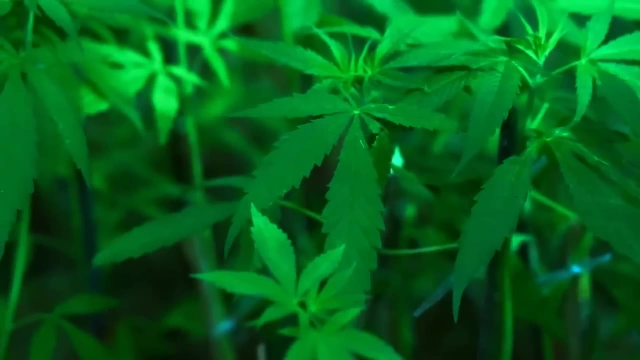 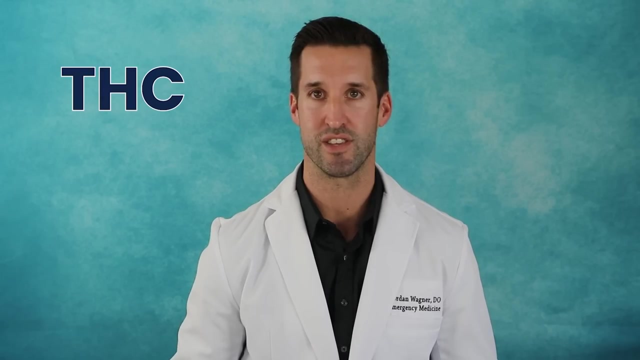 Though pea protein powder seems promising, some high quality research is needed to confirm these results. Number five, last but not least, hemp protein. Hemp protein powder is another plant-based supplement that is gaining in popularity. Although hemp is related to marijuana, it doesn't contain THC. So don't expect to get a high from a scoop of hemp in your next protein shake. okay, Hemp is rich in beneficial omega-3 fatty acids and several essential amino acids. However, it is not considered a complete protein because it's very low in levels of amino acids.